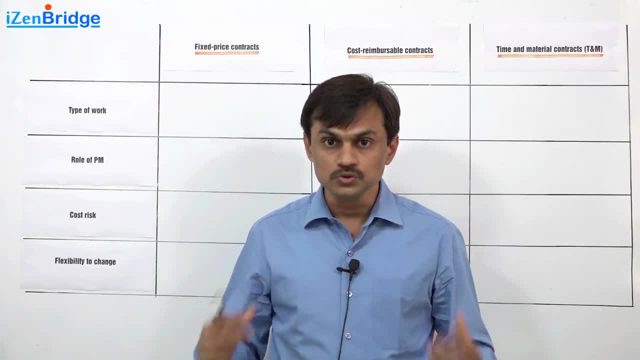 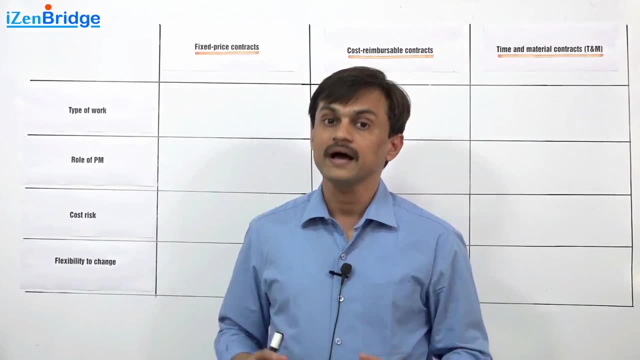 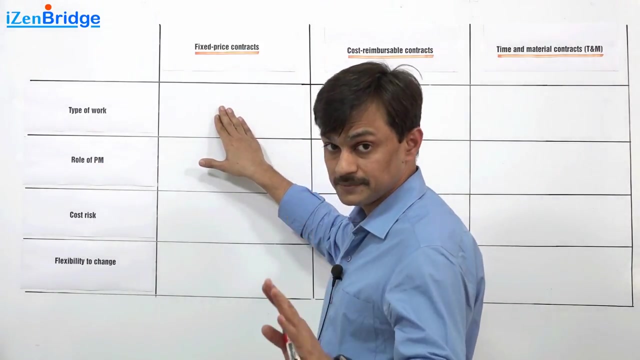 which enables buyer, No well as a seller, to do an estimation, which is, which is, which is coming in an expected accuracy range, so that both buyer and seller feel good about doing fixed price contract. so type of work where there is a more predictability, more clarity on the work examples: i spoke about flat, so you are. 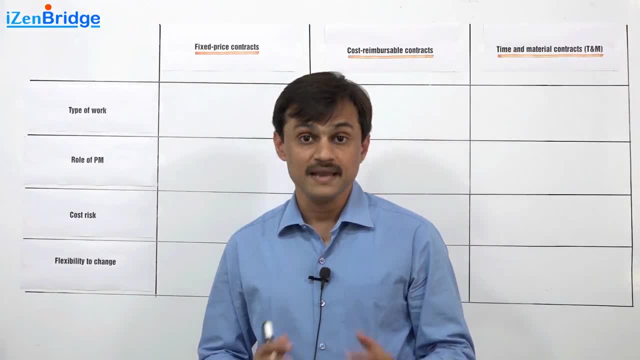 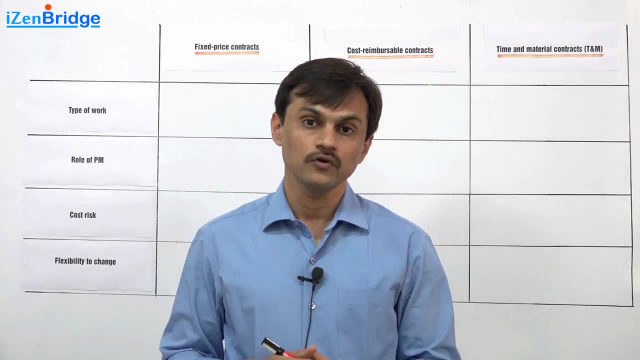 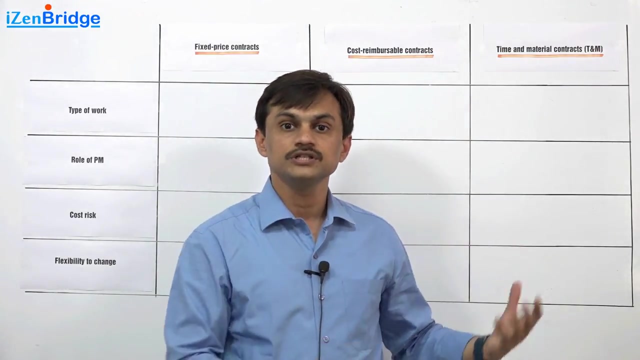 getting a flat holiday packages in software development many times when you have ready made software ready, just it requires an implementation and installation at your place. usually they go for a fixed price in engineering. when you have been creating substations for a while and another utility also want a substation, you understand you have a specification related to it. 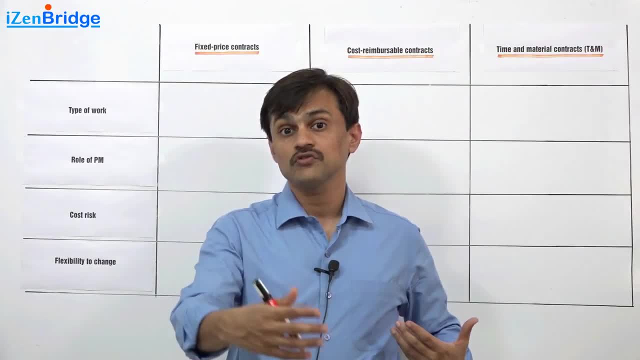 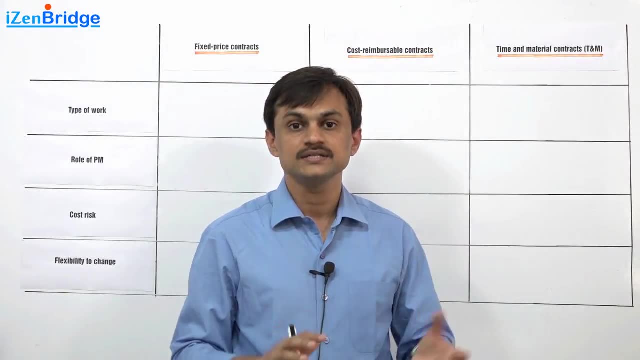 you go for a fixed price construction of a road. you have a clarity on. you have a historical data. it is not the first time you are doing. you can calculate with a decent accuracy amount of money, amount of money. you can calculate with a decent accuracy amount of money, amount of money amount. 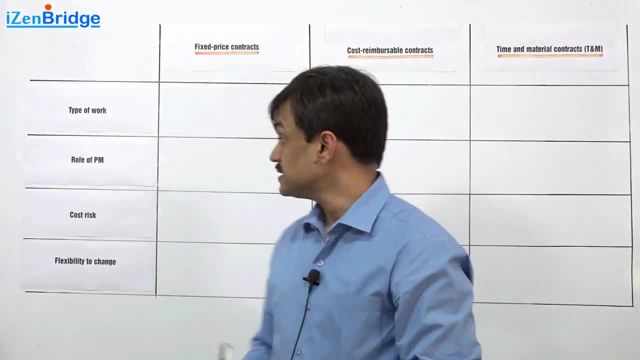 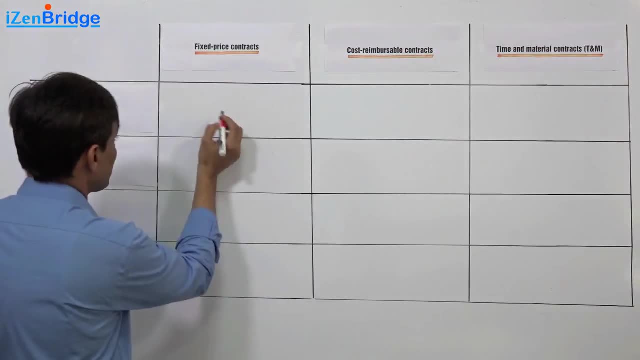 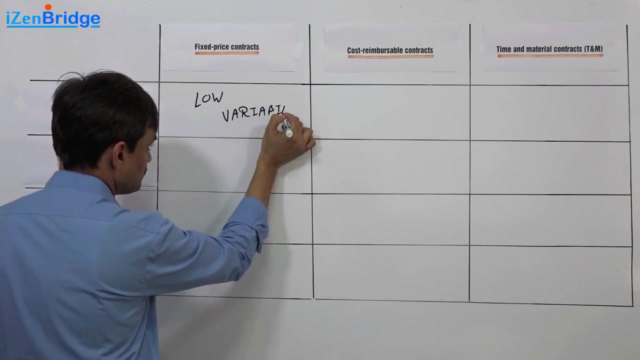 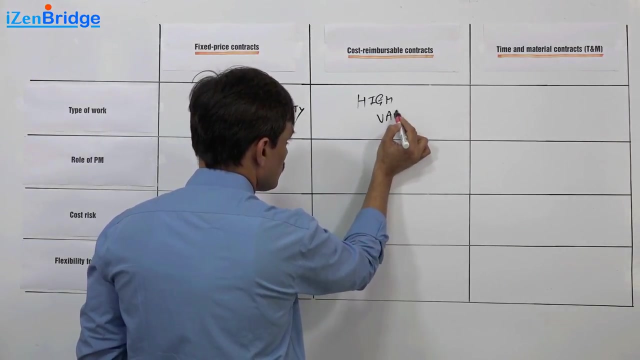 of time it's going to take. you go for for fixed price, so that's the fixed price contract cost reimbursement. so it's more like, so i can say that type of work where there is variability is low, so there is a low very ability. in cost reimbursement there is a high variability. so what does it mean? i'm just writing variable. 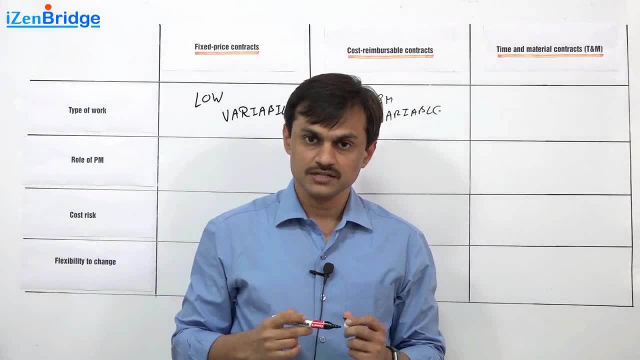 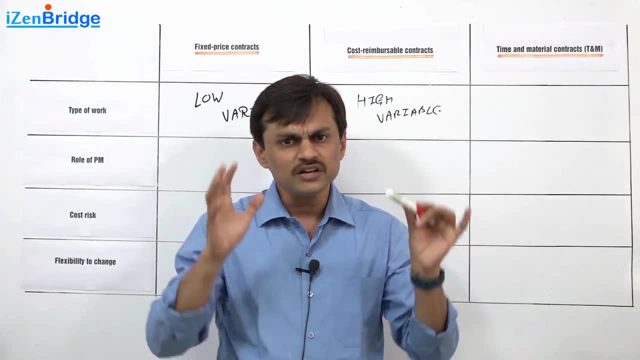 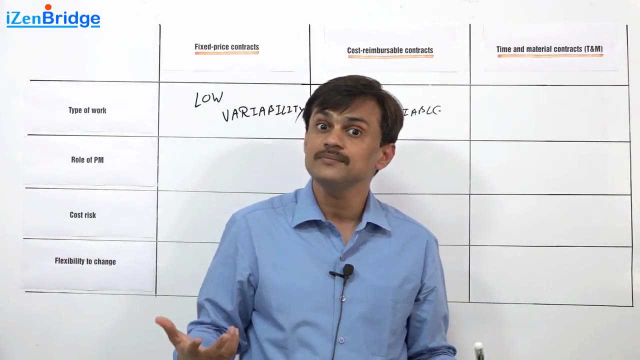 the amount of work is very much abstract. the type of the solution is abstract. the solution will evolve as we move forward. so you need something, but you don't have a pretty much clear idea of what you really want. as you see, your idea will improve and you want to definitely make use of that improved. 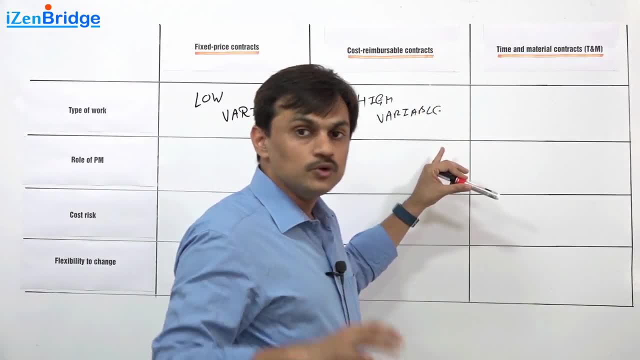 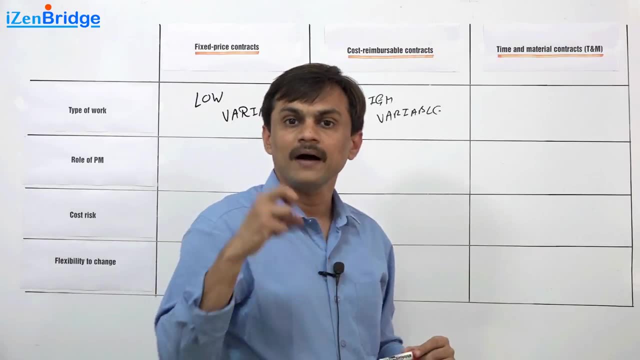 idea. when you are doing cost inversible, your goal is not to get something in a limited cost. when you do a fixed price, you primarily deals in commodities. so when you are buying vegetables or onions, or when you are buying rice grains, you know what the rice means- you have a decent idea. 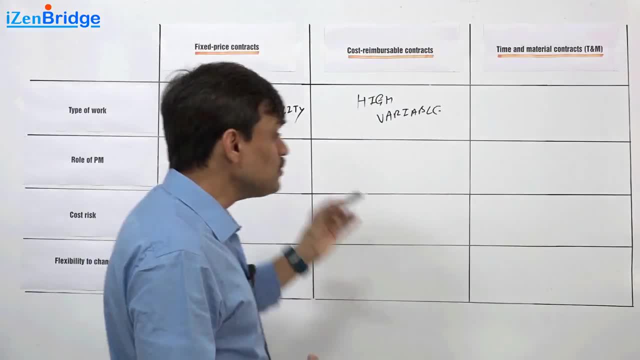 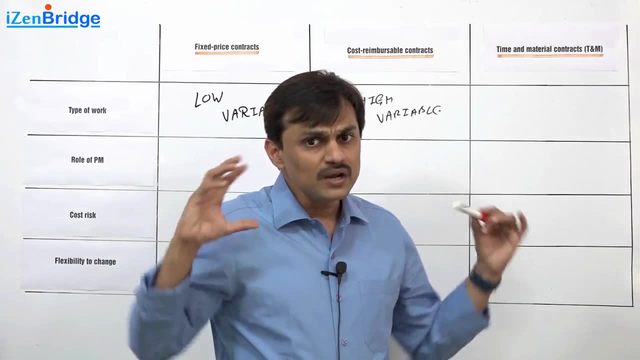 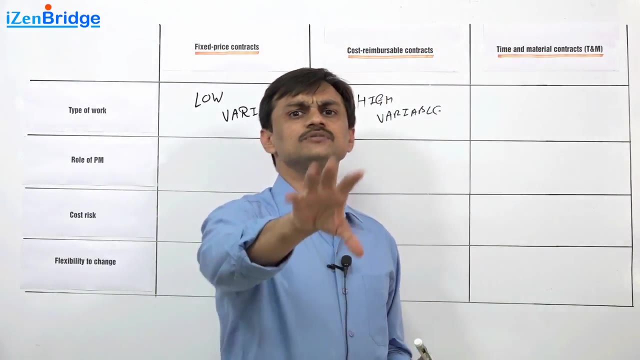 of rice and you just go for for a fixed price thing, but when you are going for creating a special dish for upcoming event or for yourself. so your idea is more focused on your goal, is more focused on creating that value, creating that experience, rather than getting something which you have already seen in a in a minimum price. so the cost reimbursement is when we get into a cost impossible contract, usually the idea of a buyer is not to get something in a bare minimum cost but to get the goal achieved, even if in between the direction changes multiple times. 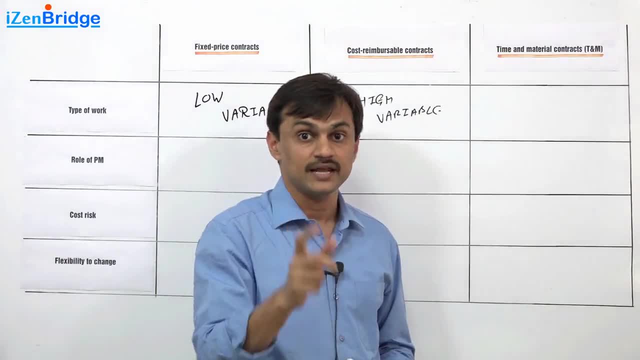 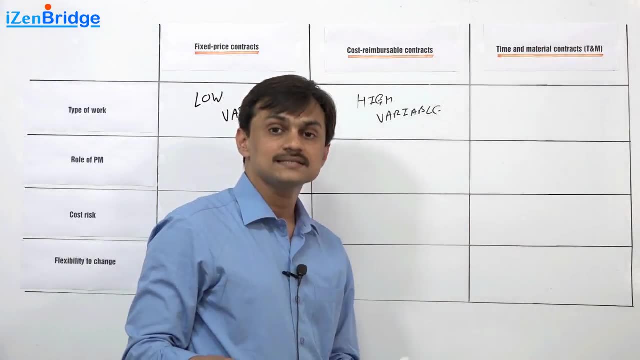 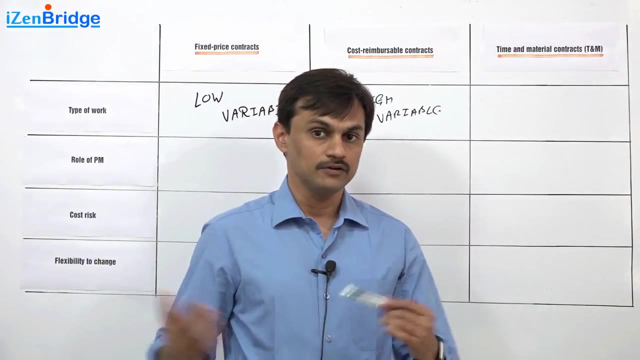 and that is why, in order to provide that flexibility of changing direction, in order to accept the variability, high variability, work goes into cost reimbursement. so, which makes the, the, the seller, also relieved that, okay, both of us are on the same boat. as the buyer is saying, i will propose the solution. if buyer likes it, i, the buyer, will pay for it. if 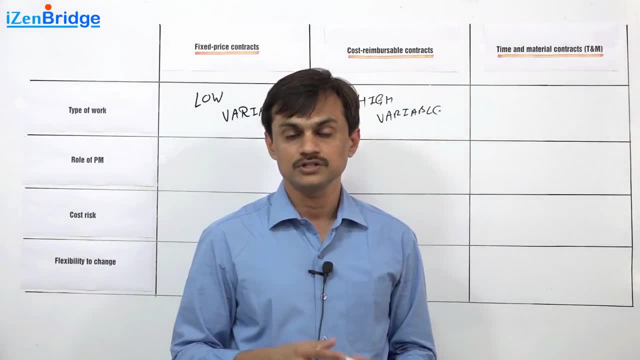 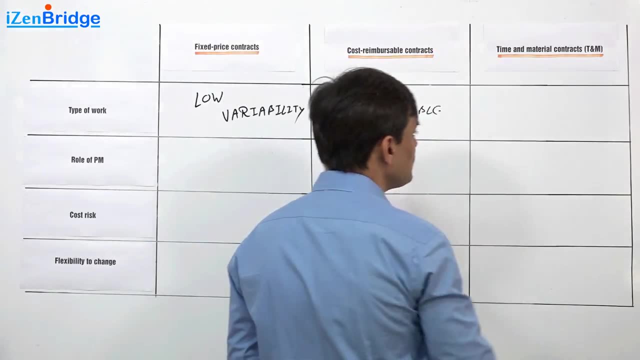 he doesn't like it, i will find another solution and this is how we will go forward. it's not like i have to implement something which is there in in my mind. so very, very high variability and, in case of a time and material, i would say a moderate variability. 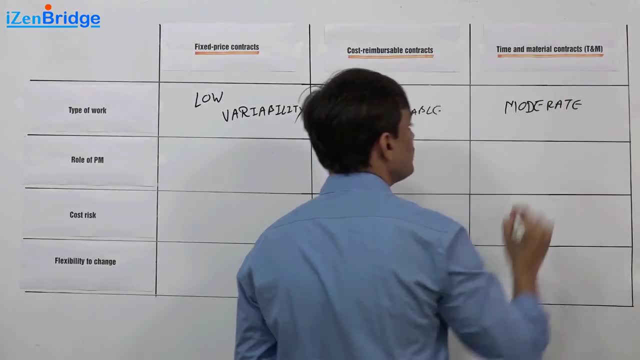 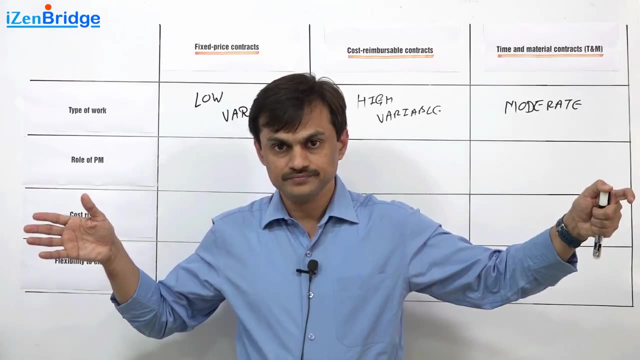 so you do have a certainty of the type of material and type of time and type of resources needed, but you don't have have a predictability of how much time it will need. so you know that there are 10 workers i want to hire. i may need it for one month, i may need it for 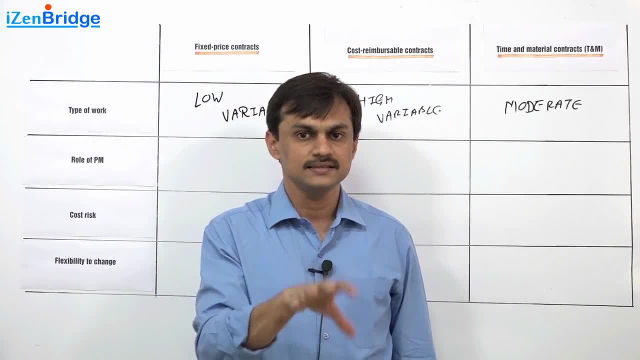 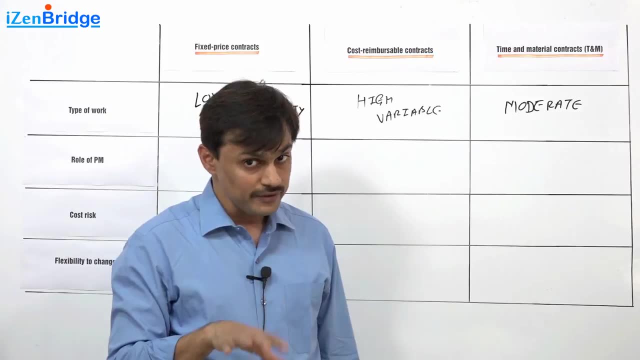 two months. but i i am clear that this is the type of skill i need and this, these guys can do that work. so why can't i have an agreement on hourly, monthly rate of of these people? so you do have a variability, but it's a moderate variability. things, at least the process, material people are pretty. 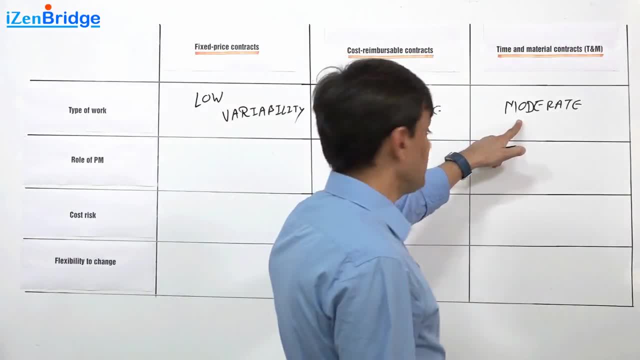 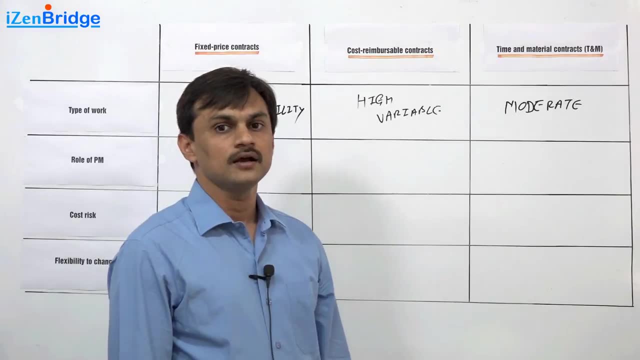 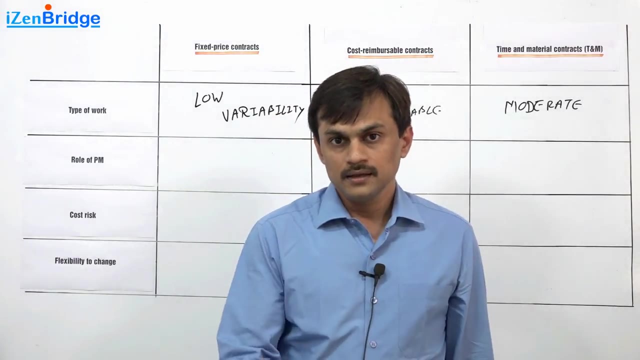 much predictable. that's why you go for a time and material based product. now, interesting thing: role of a project manager, and many time we ignore this thing. when we talk about pin box, we look at all 10 knowledge area and we we ignore the type of contract the performing organization has with the buying organization. 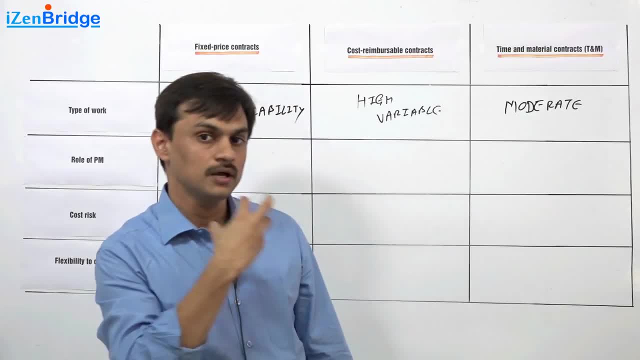 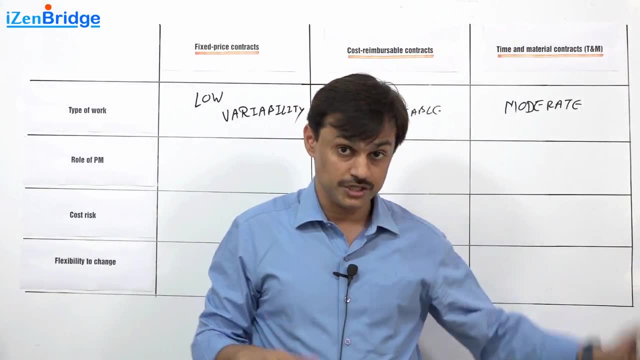 and this in case of a procurement, we are more looking from a buyer point of view. but when we talk about role of a pm, we can think of even as a project manager point of view for rest of the knowledge area. so when you are in a project manager of a fixed price contract, 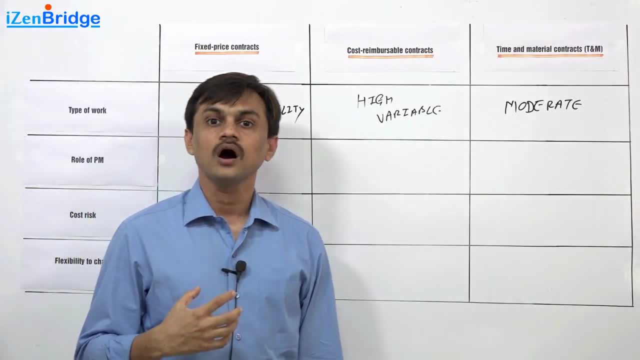 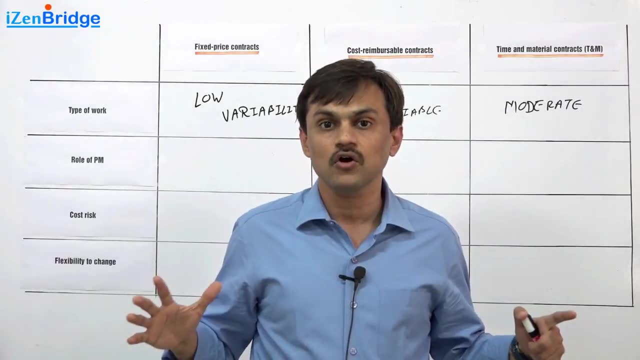 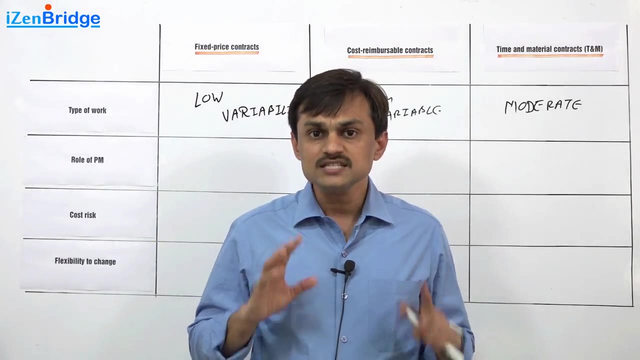 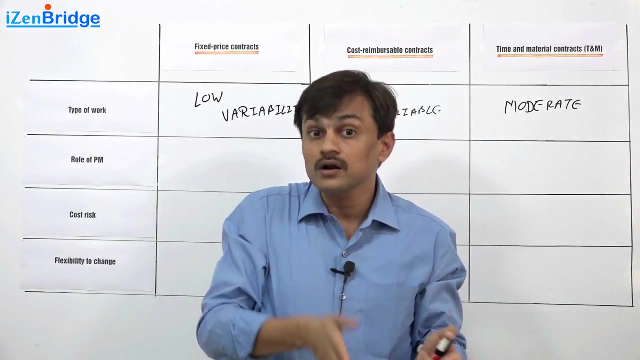 if you are managing a fixed price contract, you are managing a very accountable position. your responsibility to manage everything in a cost is very, very high. you are the one who who makes majority of decisions, because your customer does not care what kind of things you are buying. your stakeholders- the customer stakeholder- will not care about it. your sponsor will care about it. 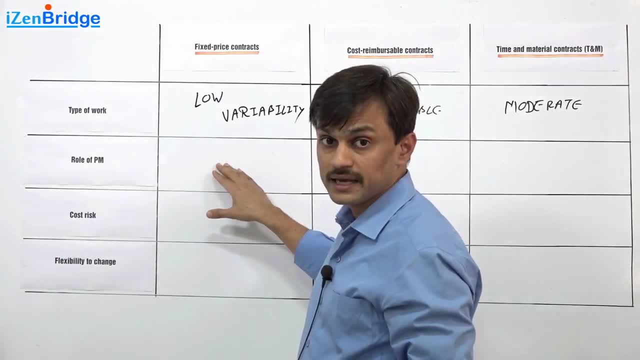 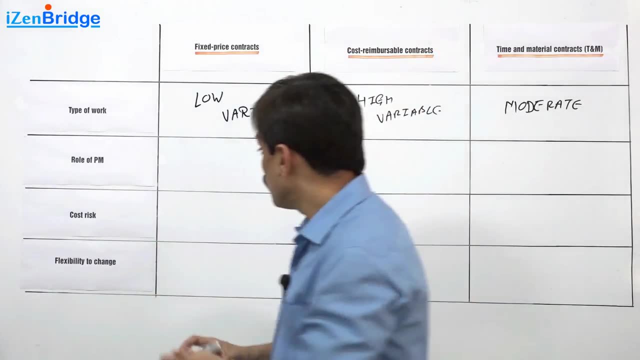 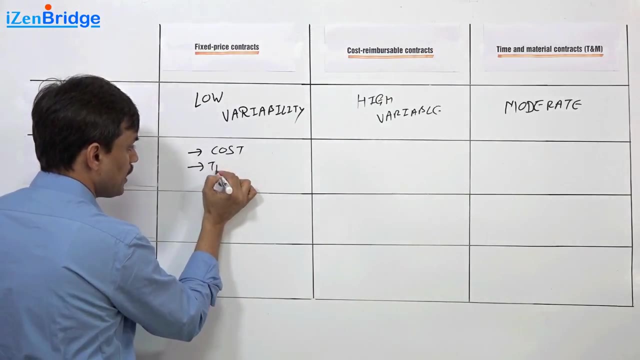 so the power in a fixed price contract, the, the project manager has full accountability of managing the project in a given price, so variance becomes too much important. so the focus on cost and time and ensuring that things happens within cost and time is is the focus of a project manager. 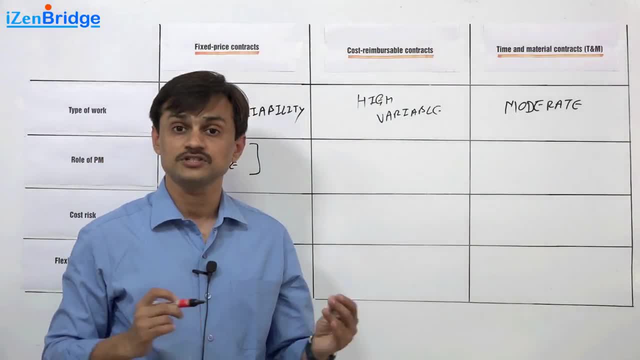 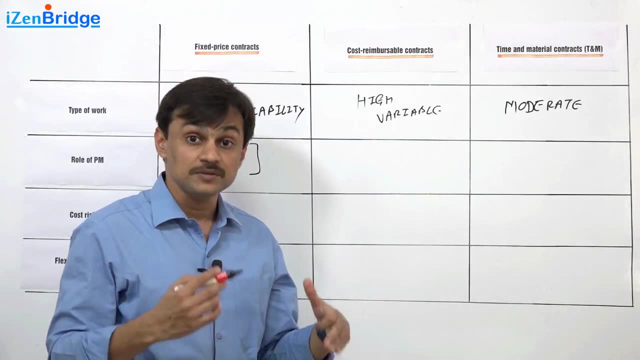 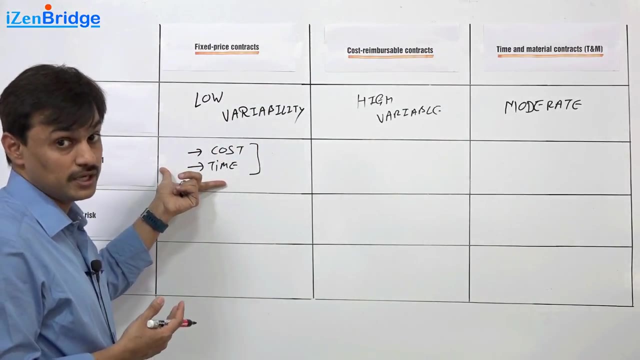 if something goes wrong, project manager end up doing escalation. project manager has to do a very refined estimation. project manager has to keep projecting the upcoming things. project manager need to do a very, very high level of risk management because this is what he has is expected to do in in fixed 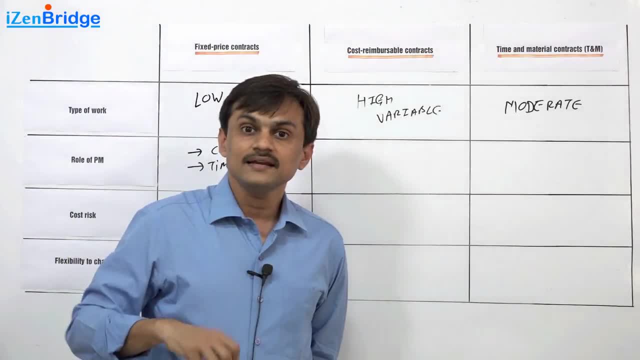 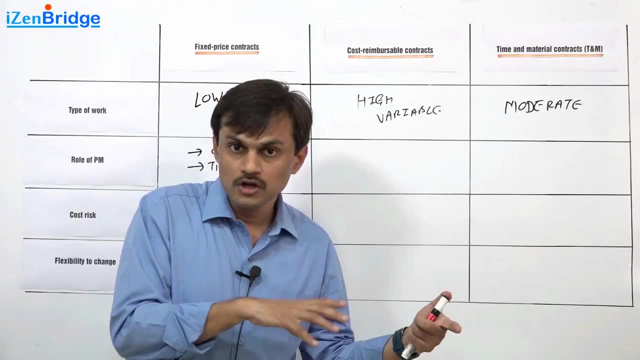 price contract, your sponsor would be targeting that how much money we can save, because we don't have committed that we will spend that much money. we only committed the work. so the sponsor focus remains that getting the work done in the minimum cost, whereas your customer- in case you, you have. 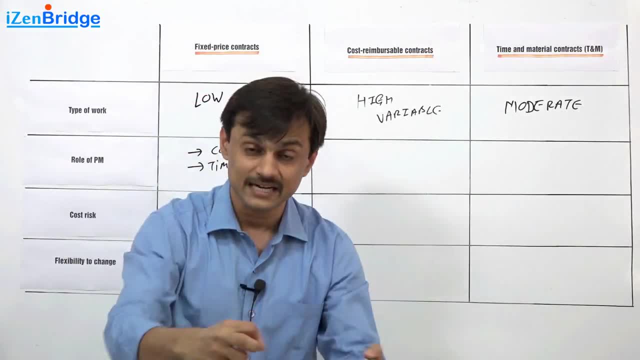 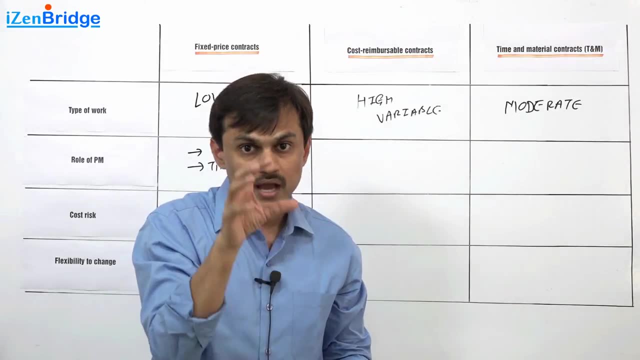 both the entities different may focus on getting what best he can get out of you because his money is fixed. now he's only focusing on what more i can get. so as a project manager you need to balance in between. you have a defined scope where customer may keep asking for more and more and more because he knows the money. 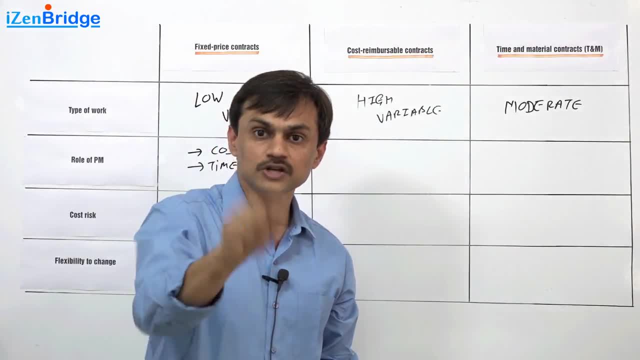 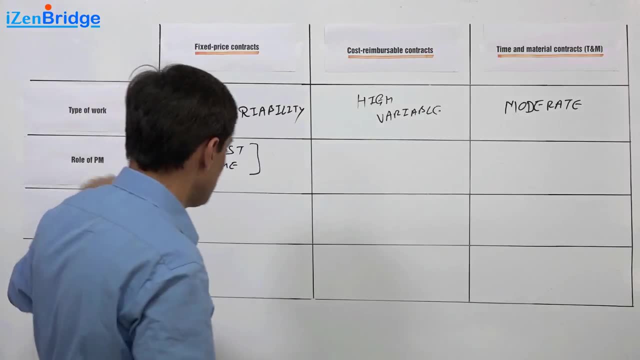 is fixed and sponsor says: if you are giving anything extra, make sure i get the money because i have taken all the risk. so that is what you see: a contradiction. when you are a project manager here, in a cost-impossible case, if you are a project manager, 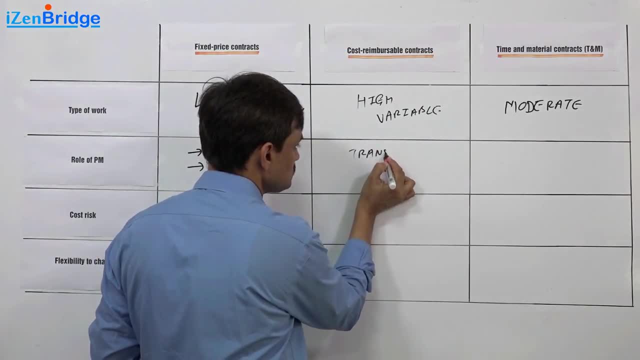 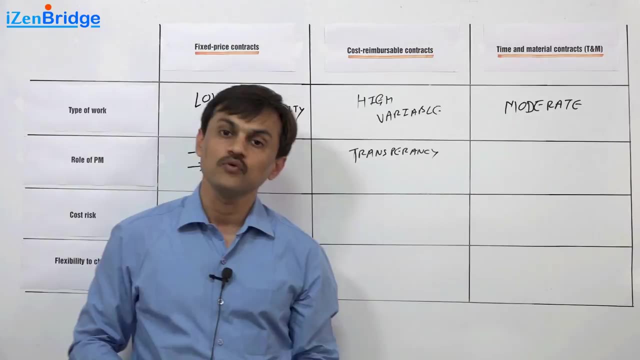 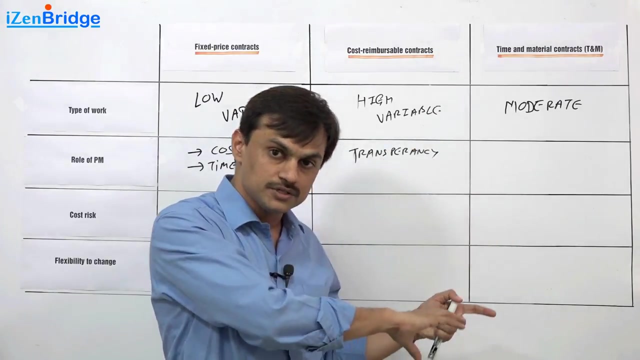 your focus becomes more on transparency. now, what is this? you need to ensure that you keep record of what you are buying, why you are buying you. you need to ensure that you have a proper history of all the approvals you take from sponsors or customers for that work, so that it doesn't happen that, without approval, you end up. 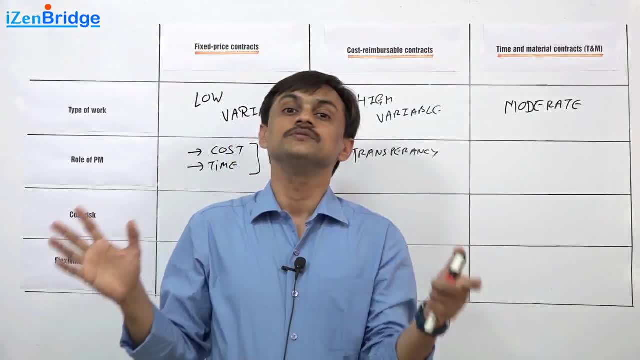 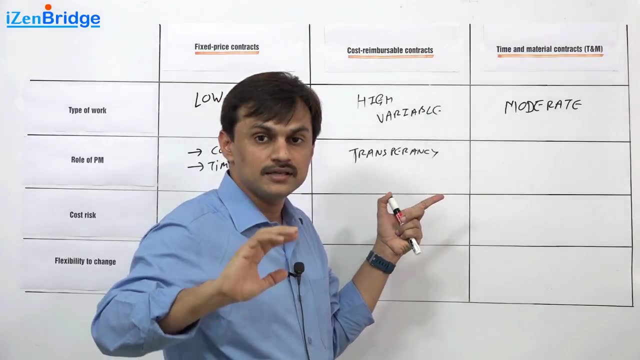 buying something and and the and the buyer says he's not going to reimburse the cost. so the focus for a project manager is to make sure that you keep record of what you are buying and why you are buying. just keep customer, keep buyer informed about everything. so buyer should be. 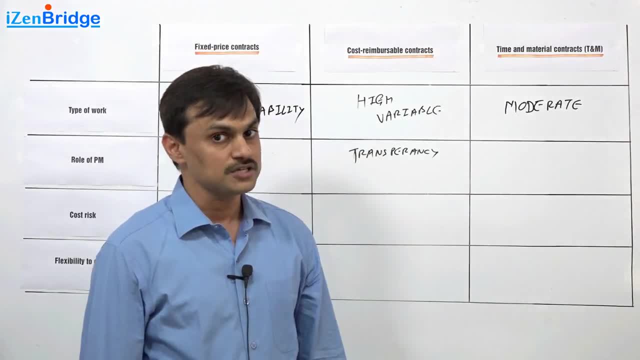 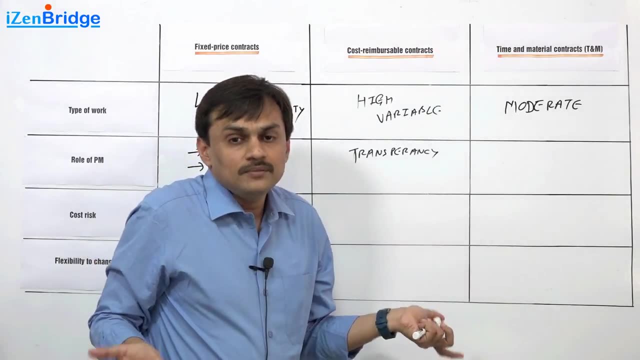 making all the decisions related to purchase and all, and your project manager should have all the signatures. that is what the project manager focuses on. if something is taking extra money, project manager has to just ensure the buyer know about it. that's it. he has not to make a decision, or we don't want to. 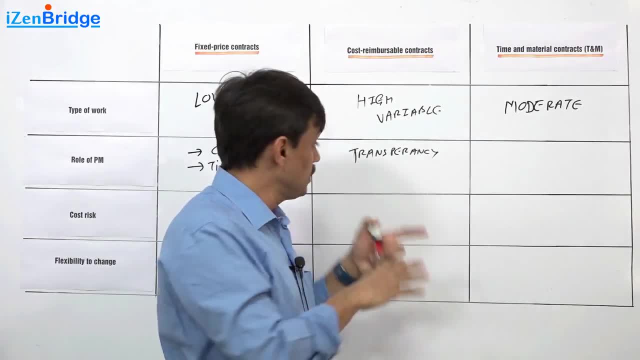 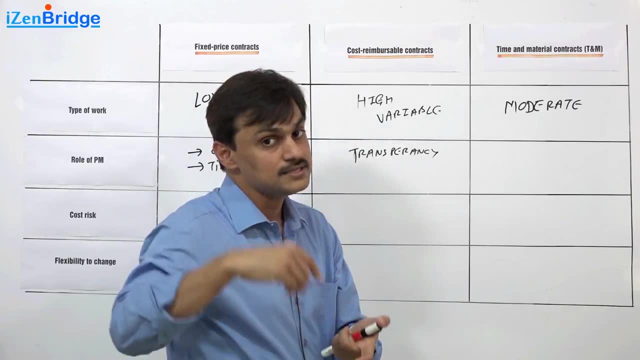 buy, we want to buy. cost variance is going high. cost variance is going low. he may. he just need to project that information to a buyer that yes, this is going beyond cost estimated. this is going like this and buyer keeps making all the decisions. so buyer is primarily responsible for managing cost and time. 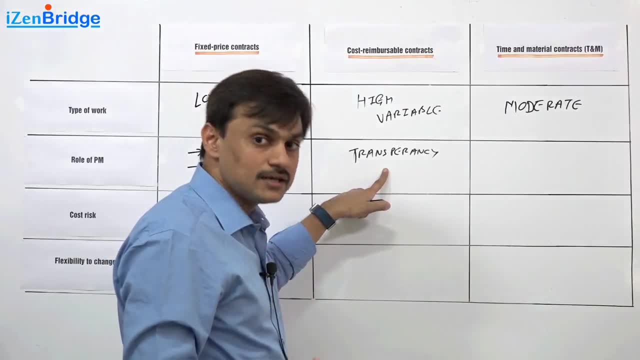 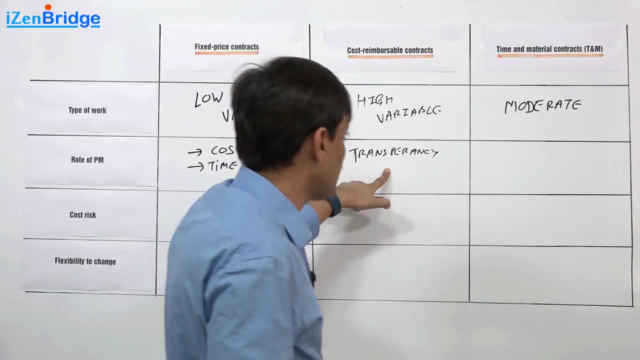 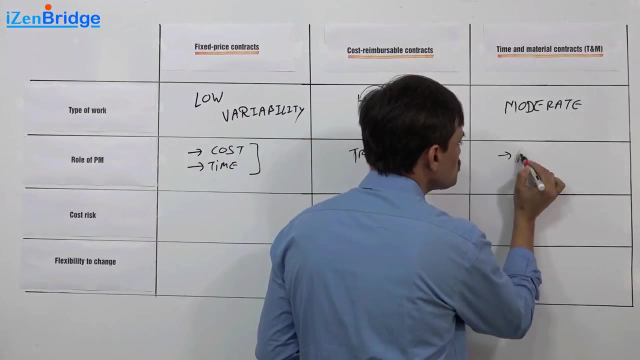 in case of cost, of cost reimbursable. as a seller, you give all the options and you make sure that all the decisions are made after taking an approval from buyer- time and material, so it's more about you need to ensure productivity. so so you show more. 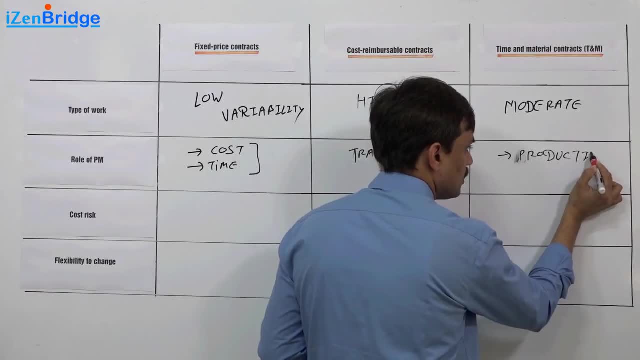 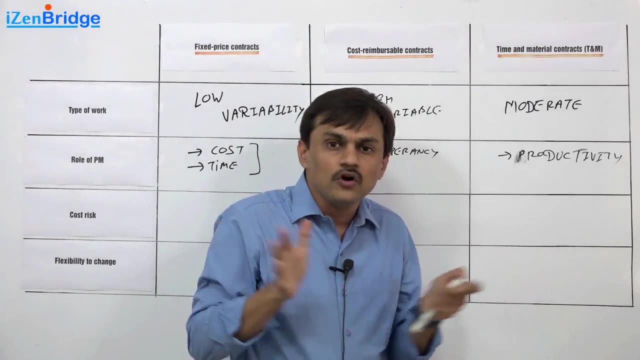 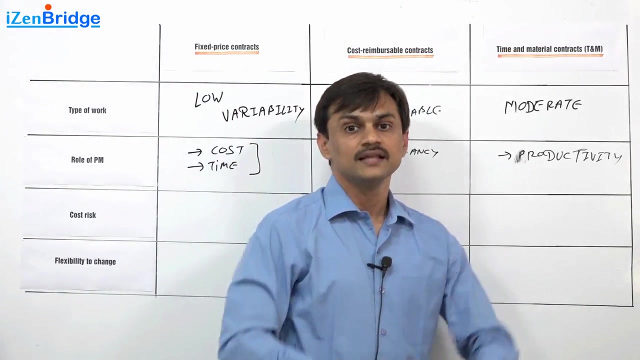 and more metrics which are driven by productivity. so it's like here also you, you don't focus too much on managing scope, managing cost and other things. you just need to ensure that people which are provided to the, to the customer, whatever time and material you have given, they are of good quality. now how? 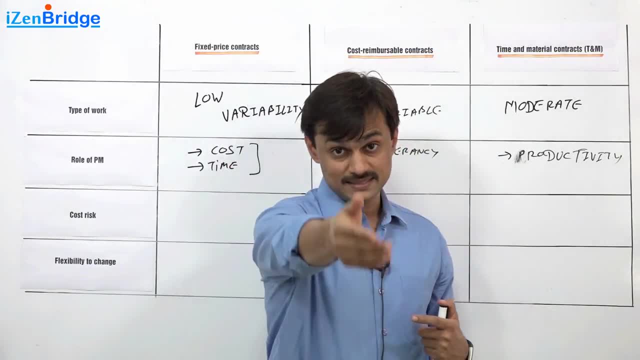 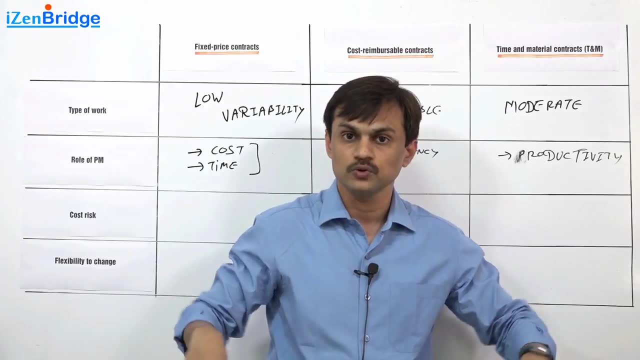 they are getting utilized is something which your buyer is deciding. so, as a project manager, if you are a seller project manager and you have given ten people to them and you are expected to manage them also, you are more and more focused on ensuring that these ten people work is. 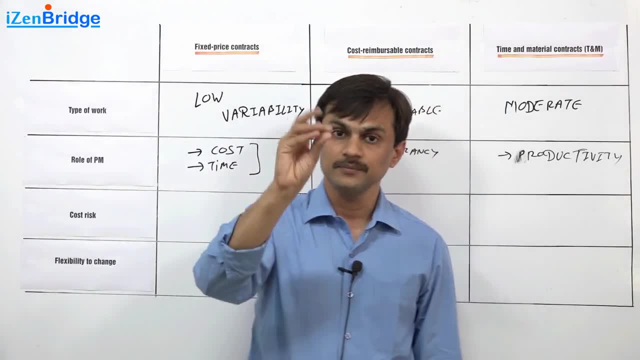 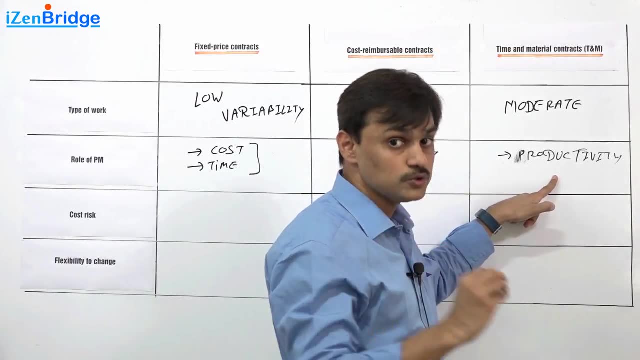 transparent. they are filling the timesheet, they are disciplined, they are coming on time and that becomes your focus. so you metrics is productivity, all those measurements is your focus area.